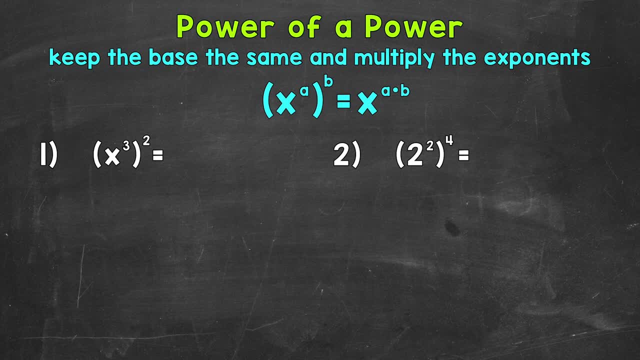 So x cubed and then we're going to square it. We keep the base the same, so let's keep our base of x here. And then we multiply the exponents, so 3 times 2. That gives us 6.. 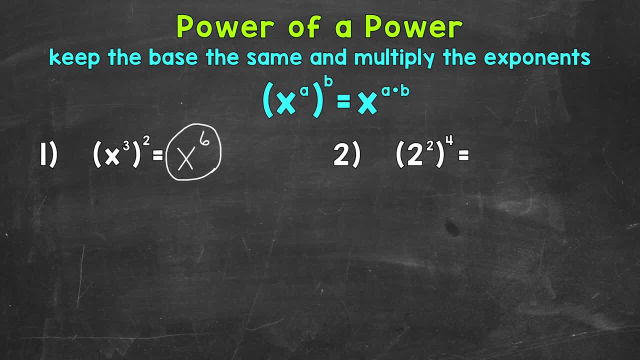 So our solution is Now: let's break this down and see exactly how it works. So x cubed and then we square it. So let's square x cubed. That means we have x cubed, or x to the power of 3,. 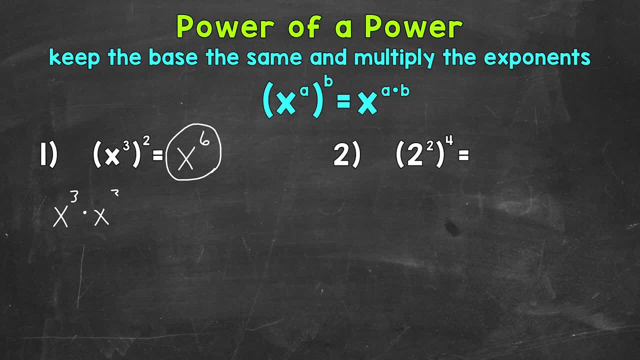 times x cubed. Let's break it down further: x cubed, well, that means x times x times x. So we have x to the power of 3 times x cubed. So we have x cubed over here: x times x times x. 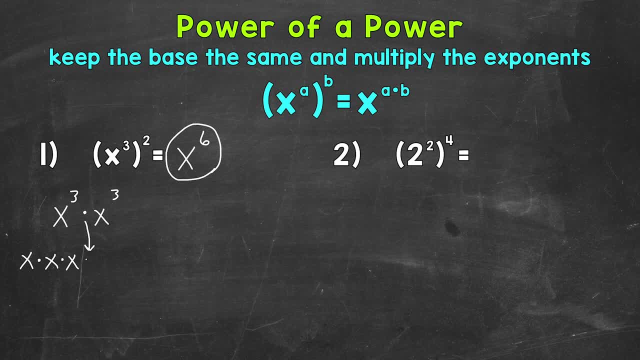 And then let's bring our multiplication sign, that's in the middle. bring that down. And then for the other x cubed, that means the same thing: x times x times x. So we have an x cubed right here, And then we have an x cubed right here. 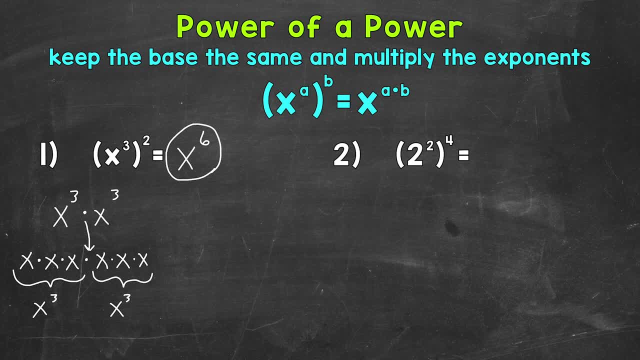 We have 6.. And then our next problem is our total x, which is x to the 6th power. So you can see how everything works out after we break it down. So keep that base the same And then multiply the exponents. 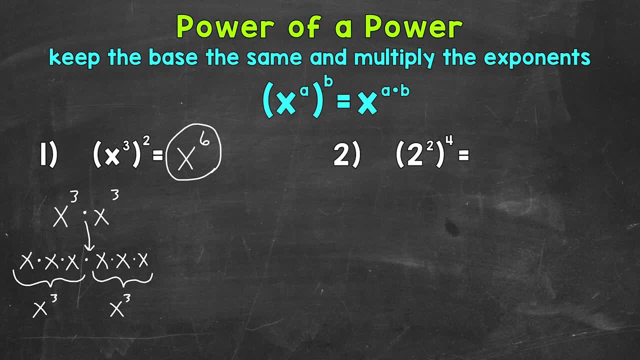 Let's try another example and move on to number 2, where we have 2 squared to the power of 4.. So keep the base of 2 the same And then multiply the exponents, So 2 times 4, that equals 8.. 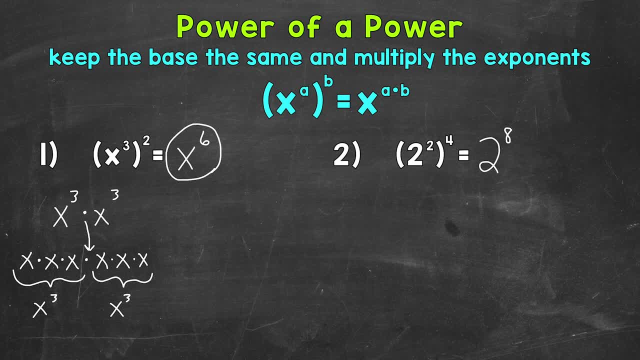 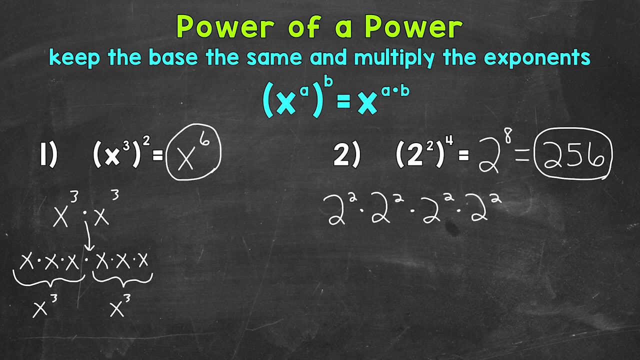 so we get 2 to the power of 8. for our solution. now that equals 256. let's break that one down as well. well, 2 squared to the power of 4, that means 2 squared times 2 squared times 2 squared times 2 squared. let's break it down further: 2 squared means 2.